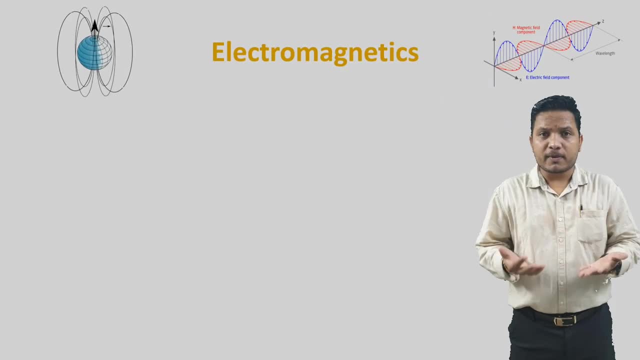 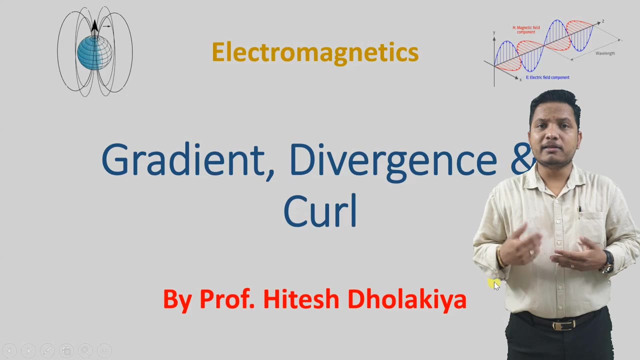 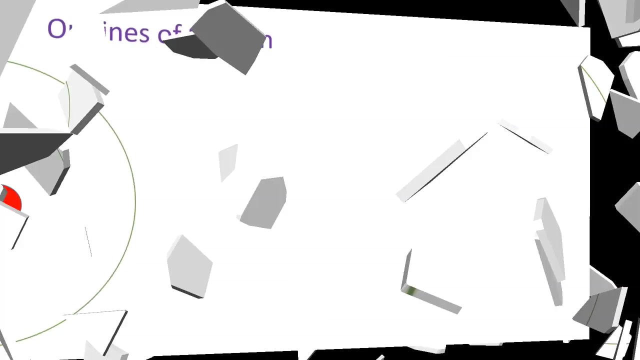 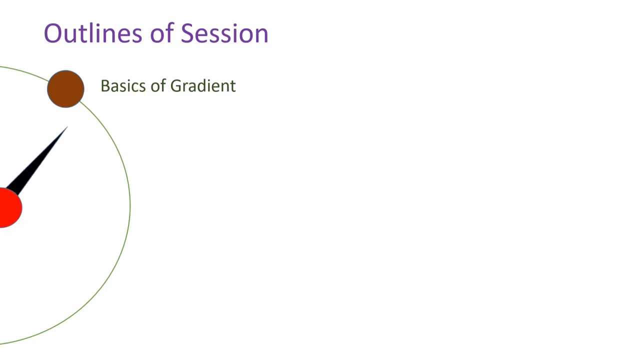 Welcome to Electromagnetics playlist I. Professor Hitesh Dulakia is going to explain you gradient divergence and curl in this session. So to understand gradient divergence and curl, these are my session outlines. So first I will explain basics of gradient and then we will solve. 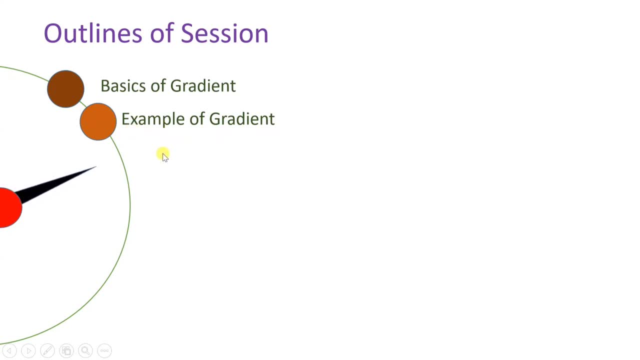 one problem based on gradient. After that I will explain basics of divergence and from divergence we can have divergence theorem. and then, based on divergence, we will solve one problem. Then, after, I will explain basics of curl and based on curl we can calculate stocks theorem. 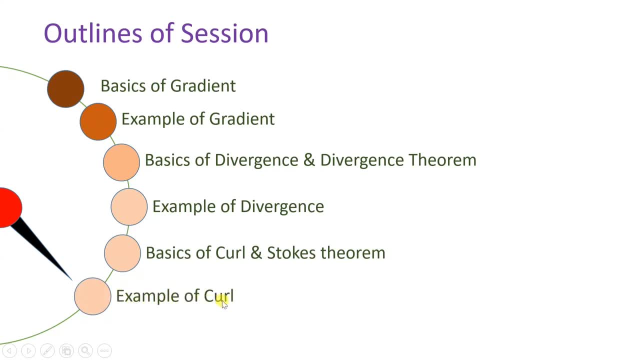 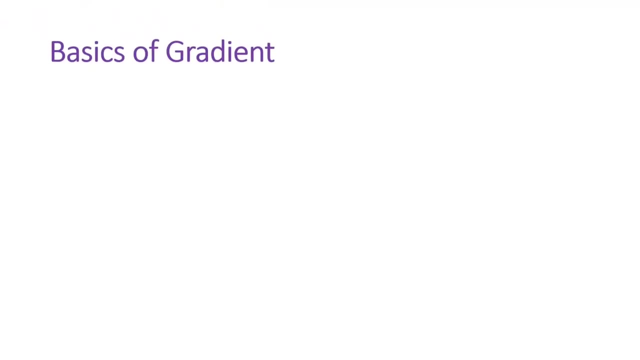 and then I will give you one physical explanation of meaning of curl. So all those things that will be the case, which I will explain in this session. So let us begin this session with first agenda, that is, basics of gradient. Now see, before I initiate with this session, we should know what is del operator. So here, 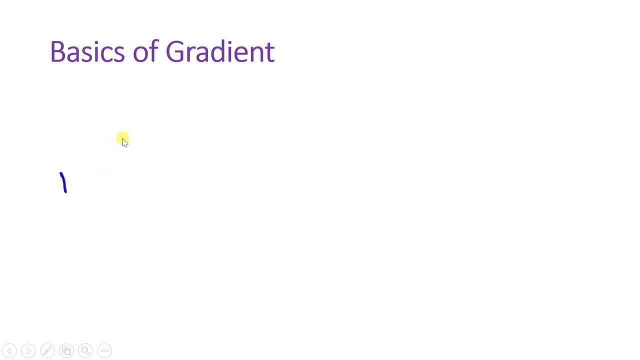 I am writing it: See del operator. so that is a vector operator and meaning of del operator, that is, del by del x of i, I plus del by del y of j plus del by del z of k. Why am I telling this? the reason is ingredient in divergence and in curl. 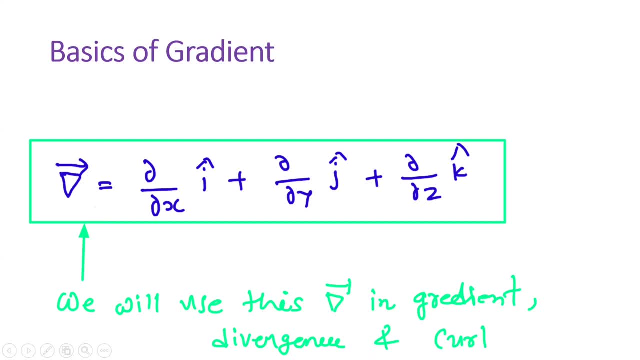 we need to apply that del operator So this del operator that we are dealing with, to apply that ingredient divergence and curl, So del operator is vector operator And that is del by del x of i plus del by del y of j plus del y del z of k. Now let us start this session with gradient. 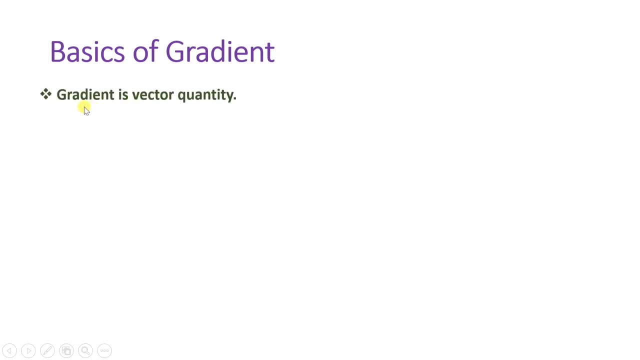 So gradient, that is a vector quantity. So resultant after calculation of gradient will be a vector quantity and gradient is applied to scalar quantity. So function on which we apply gradient will be a scalar quantity. So let us try to understand that by functions. it will be more clear. See gradient of f, where f is scalar quantity and del operator that. 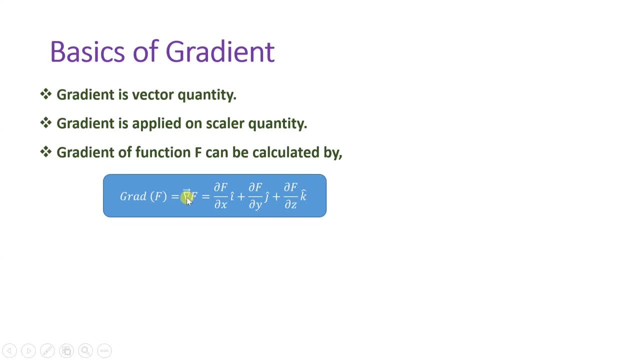 is a vector quantity. So gradient of f, that is del f and that will be vector quantity. that will be del f by del x into i, plus del f by del y into j, plus del f by del z into k. See, this is how gradient will be there Right. And when you try to understand what 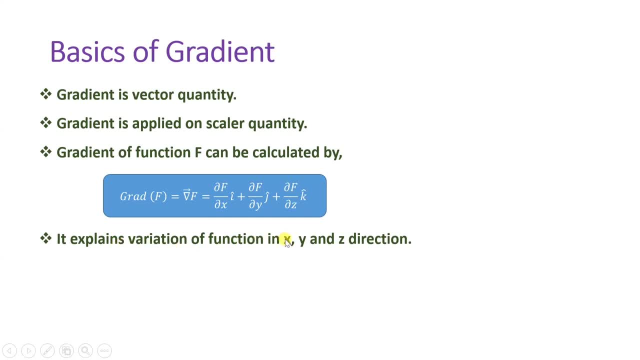 is the meaning of gradient. So that explains variation of function in x, y and z direction. Like see, when you have one scalar function. let us say we have a room in which we turn on our air conditioner system. So when you turn on air conditioner system in a room, 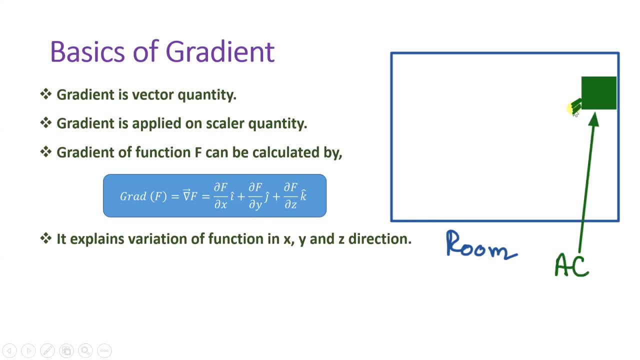 here I am placing AC, So once you turn it on you'll be finding the region nearer to to air conditioner will be getting cool very fast, and the region which is far from the air conditioner will get cool bit slower. right, so the variation of temperature in entire. 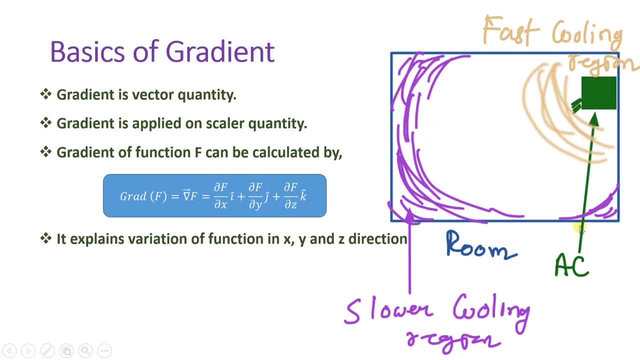 room that is based on position and that variation that we can understand by having gradient. why? the reason is temperature is a scalar quantity and by having gradient we can understand how temperature varies with respect to x, y and z direction. so this is one practical example. so, for example, if we apply gradient to a function of temperature, then from gradient we can understand. 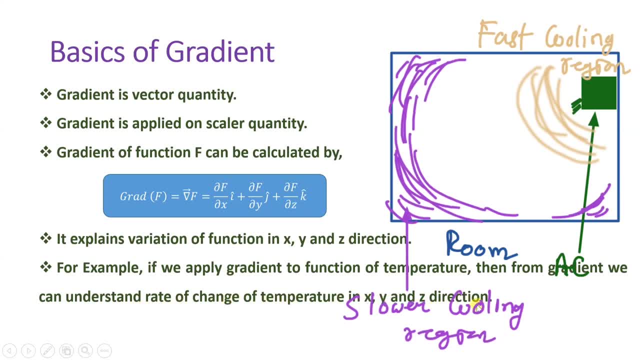 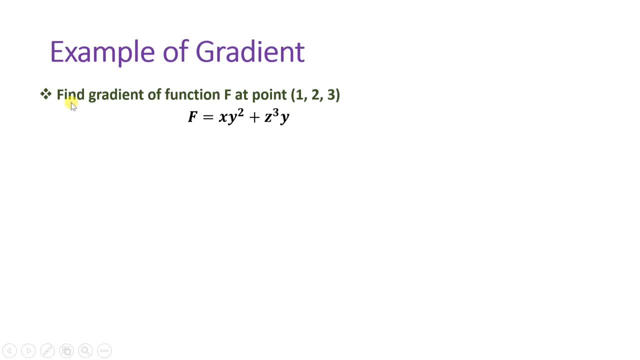 rate of change of temperature in x, y and z direction. now I will explain you one example so it will be more clear. See, the question is: find gradient of function f at point 1, 2, 3, where function f is scalar function, and that is x, y square, plus z, cube, y. now, as we know, gradient of f, that is del f, that is: 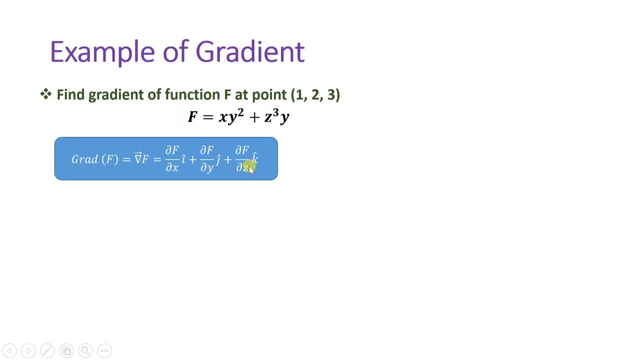 del f by del x i plus del f, by del y j plus del f by del z k, and where f once you apply that, so that will be x, y y square plus z cube y. that is f. and if you do partial differentiation over here, then 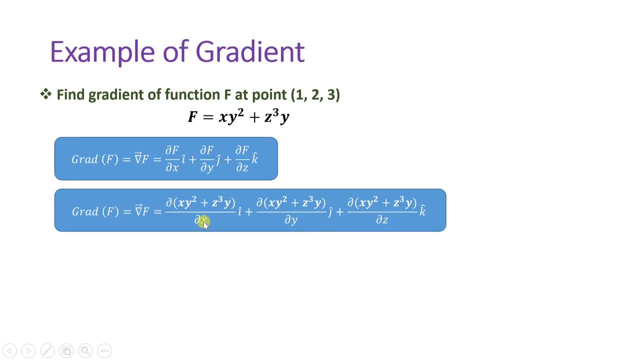 over here you can see. see, this is what del by del x. so partial differentiation with respect to x. so this x will be 1 and y square, and this is constant. so this will be 0. so resultant of this much is y square. now, here, partial differentiation with respect to y is there. 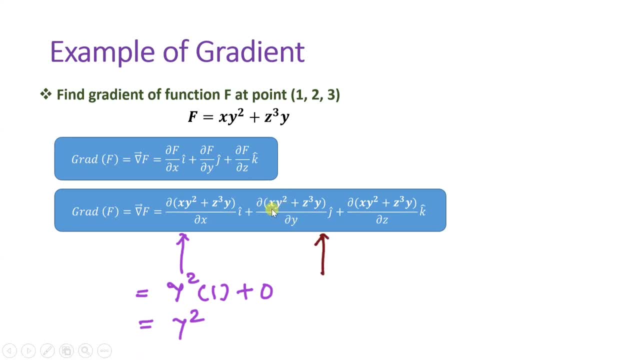 so x is constant. y square is having 2 y, so 2 y x plus z cube into del y by del y that is 1, so 2 y x plus z cube. that is what resultant of this and for partial differentiation with respect to z over here, x y square, that is constant, so it's z, it's partial differentiation. 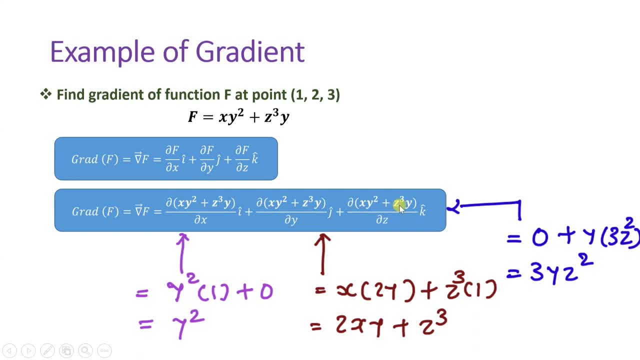 is 0.. z cube, That is 3 z square and y is constant. so resultant of this will be 3 z square y. so you can see, for this it is y square, for this it is 2 y x z cube and for this it is 3 z square. 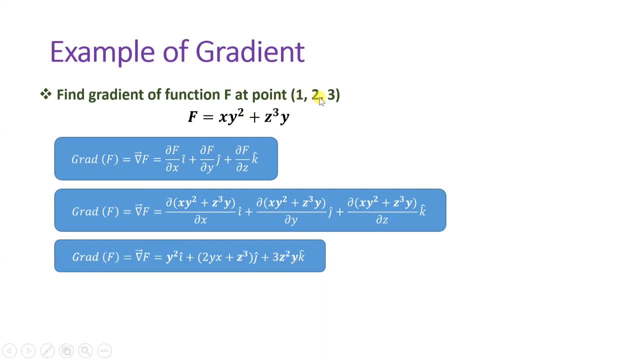 y. now at this point, 1 comma, 2, comma 3, if I want to calculate this value of gradient, then you can see y square where y is 2, so y square is 4, so 4i. plus this 2yx plus z cube: where y is 2, x is 1, so 2, into 2, 4, z cube. so 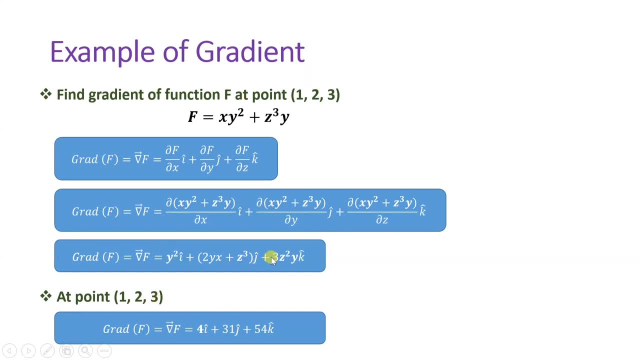 3 cube, that is 27 plus 4, that is 31, and 3 z square y, so 3 into 9, into 2, so 18 into 3, 54.. So this is how we have gradient of function f. So we can see clearly at this point with respect. 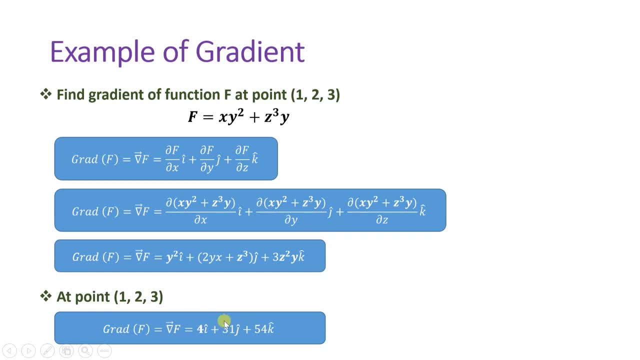 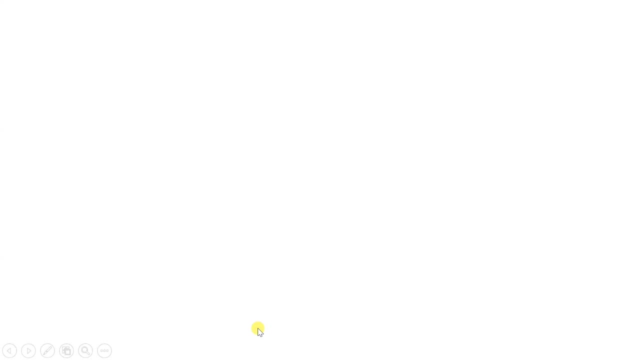 to x, coordinate variation is 4, with respect to y, coordinate variation is 31 and with respect to z, coordinate variation is 54.. So this is what the basic meaning and calculation of gradient. Now I will explain you basics of divergence. Now see, divergence is a scalar quantity and we apply divergence on vector quantity. 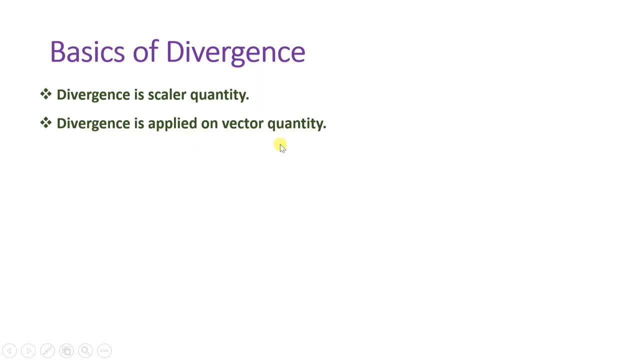 So divergence is a scalar quantity and we apply divergence on vector quantity. And whereas we have seen gradient in previous slide, where gradient is a vector quantity and we apply that on scalar quantity, right, While here divergence, that is, vector quantity, is a scalar quantity and we apply that on vector quantity. 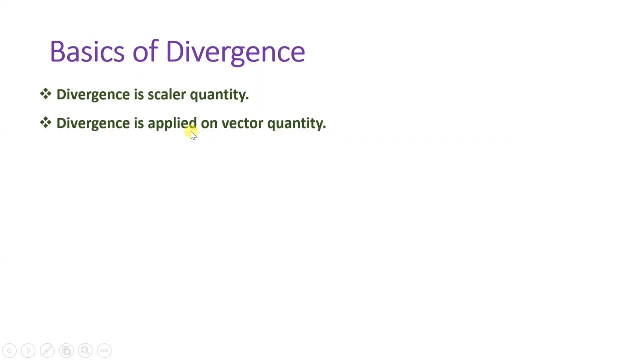 So we have seen gradient in previous slide where gradient is a scalar quantity and we apply that on vector quantity. Let us see that in with respect to function. So see divergence of f. that is del dot f- See previously. gradient was del f, while divergence is. 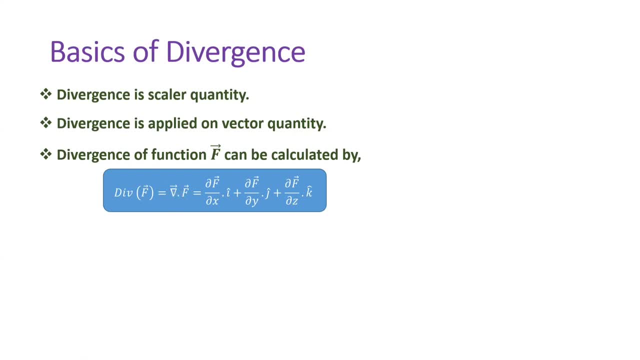 del dot f. That is the basic difference which is there in between divergence and gradient. Now, see here, all we need to do is we need to have dot multiplication, Right. So dot multiplication, that we need to do. So here, see del vector f by del x dot i, plus del vector f by del y dot j, plus del vector f by del z dot k. 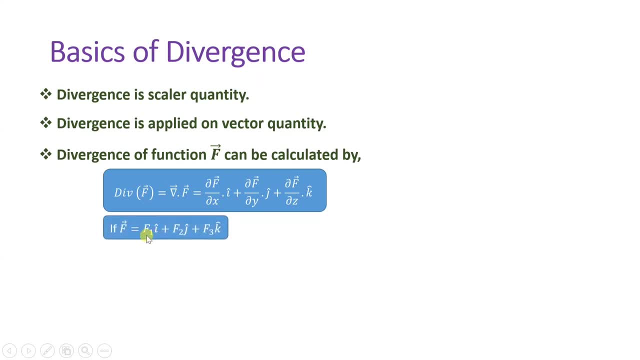 Now here, if I say we have vector f, that is f1, i plus f2, j plus f3, k. So in that case, see this dot multiplication That will be happening with respect to i coordinate, j coordinate and k coordinate. So here, resultant of this term, that will be del f1 by del x, plus resultant of this term, that will be del f2 by del y, plus resultant of this term, that will be del f3 by del z. 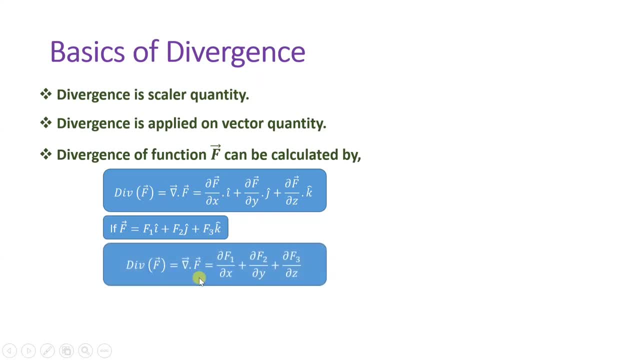 So you can see Now divergence, that is del dot f, that is partial differentiation of x, component of function, with respect to del x, plus partial differentiation of y, component of function, with respect to del y, plus partial differentiation of z, component of function, with respect to del z. 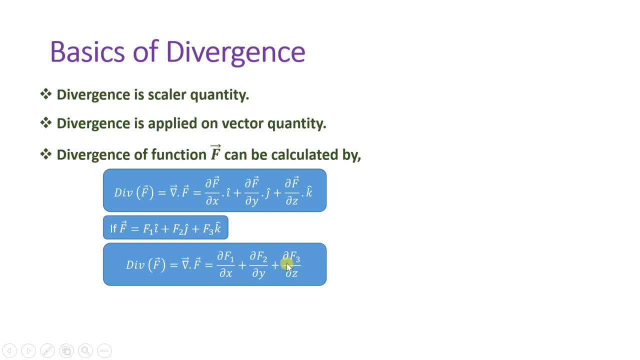 See, this is how divergence is getting calculated. Now we need to understand what is the meaning of divergence. So see, there is one more way by which we can calculate diversion, See del dot f. that is diversion, and that is equals to limit. volume tends to 0. surface integration of function divided by volume. 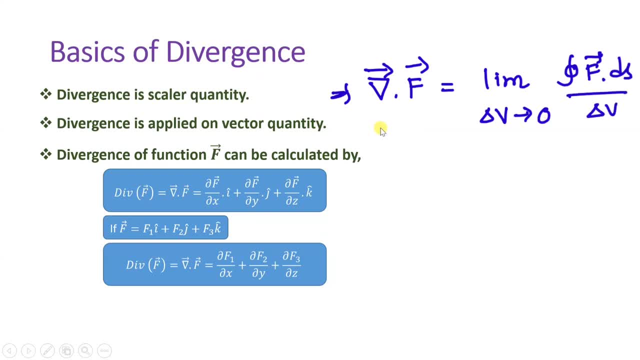 So from that we can say volume. So volume integral of divergence is equals to surface integral of function. So volume integral of divergence is equals to surface integral of function. So here we have a relation of volume integral and surface integral, and that is what divergence theorem. 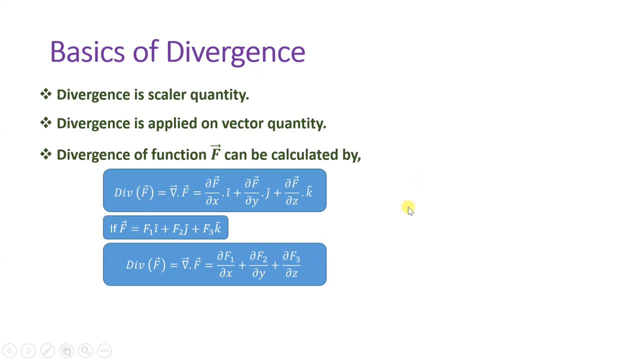 I will explain this by one example, so it will be more clear. So see, it explains overall variation of function In x, y and z direction. Now see to understand that. I will explain one example, so it will be more clear. Now see, here we have a tank and in that tank, by this pump, we pour a water inside. 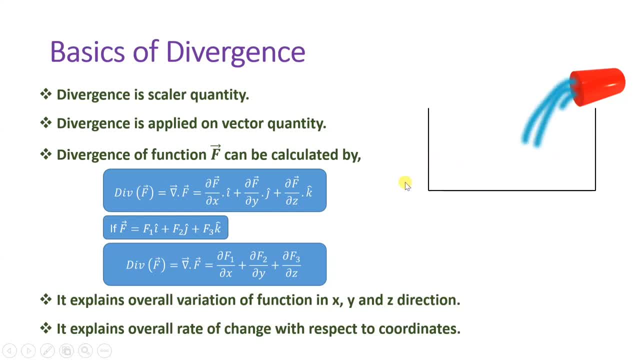 So water is coming inside in this tank. Now see here if I have some valves and if I open these valves. So So what will happen? rate of change of water at this position, that will get decrease and water that is actually getting pour from this main pump and it is coming first over here. 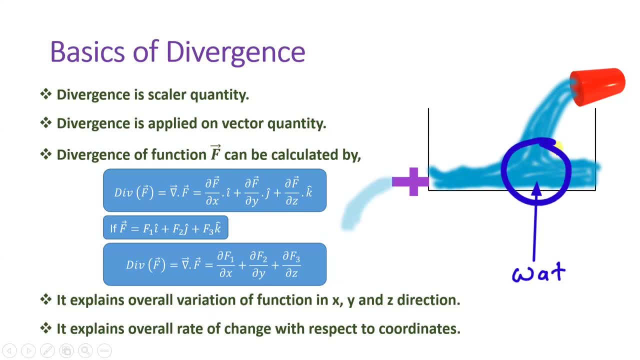 So you will be finding water is more over here. So water change that is increasing over here. over this side you will be finding water change is constant. over this side You will be finding water change is decreasing. So we can say Divergence of water change over here. that has to be negative. 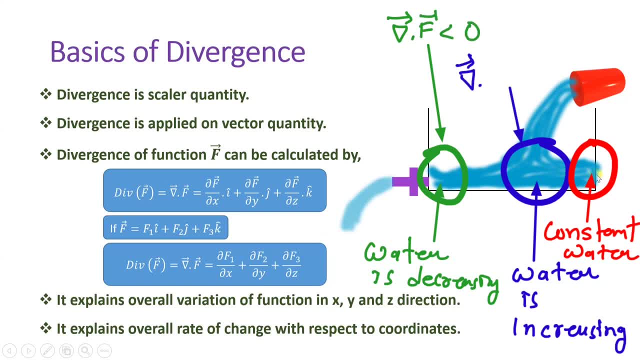 Divergence of water change over here, that has to be positive, and divergence of water change over here, that should be zero. Why the reason is: over here water change is not happening. So this is what the basic meaning that one can understand, based on divergence theorem. 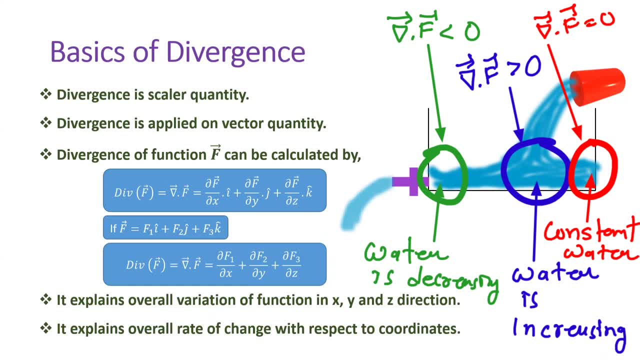 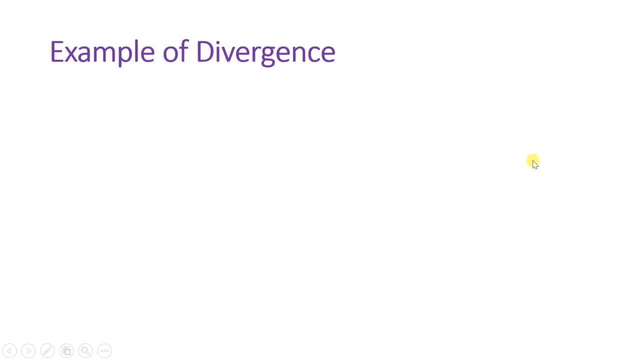 So it explains overall rate of change with respect To co-ordinates. so let us try to understand that by one examples. it will be more clear See. Question is: find divergence of function f at point one, two, one and this function is vector function. as we know, divergence should get applied on vector quantity and the resultant of divergence, that is, a scalar quantity. 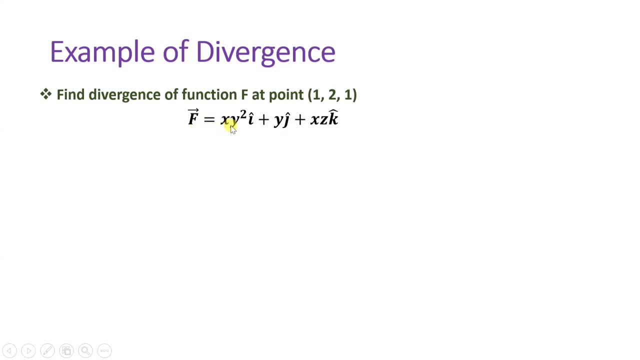 So here, vector f, that is this x, y square, i Plus y, j plus z, X, z, k. Now, As we know, divergence of function, That is, del f, one by del x plus del f, two by del y plus del f, three by del z. 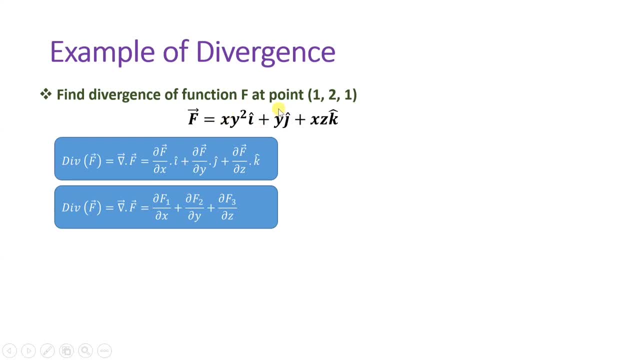 Where f one, that is i coordinate, f two, that is j coordinate and f three, that is k, coordinate Right. So f one, that is x, y square and that we differentiate with respect to x, So partial differentiation of this, that will be y square. 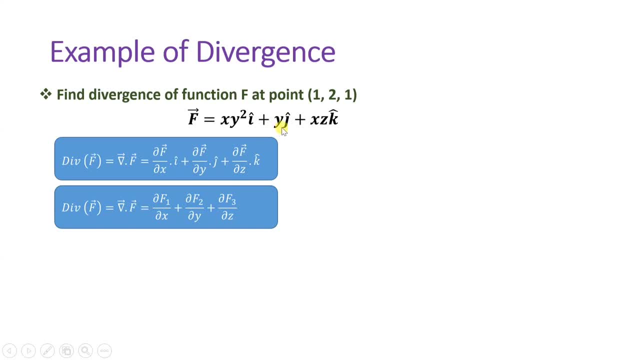 For this del f two by del y, here this is y, so del y by del y, that is one. And for this third coordinate del f three by del z, where f three is x, z, so x is constant. del z by del z is one, so this will be x. 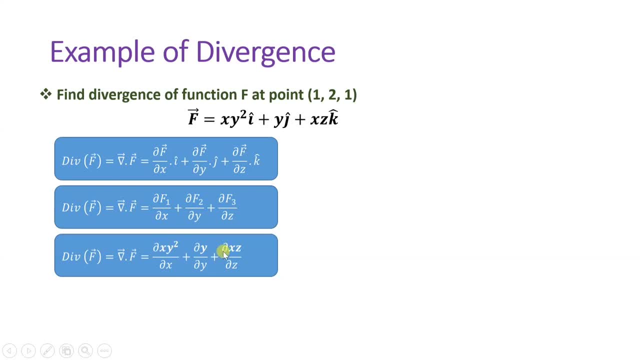 So divergence of this function. If you do this you'll be finding that is y square plus one plus x. So here at point one, two, one. If you place the values where y is two, x is one, so that resultant will be six. So we can say: divergence of this function is six. 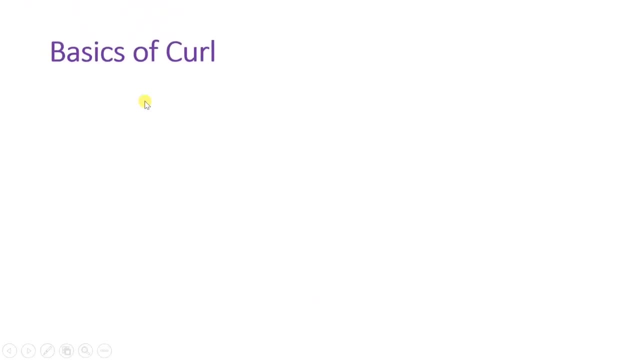 Now I'll explain curl, So basics of curl, that we will discuss first here And then we will see the practical example based on curl. Now see, Curl Is a vector quantity And curl is applied on vector quantity. See, initially we have seen gradient, so gradient is vector quantity. we apply that on scalar quantity. 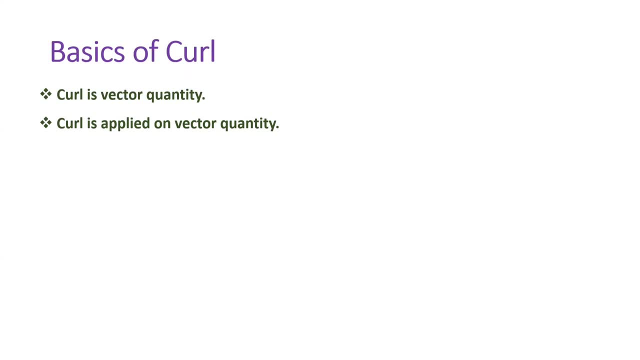 Divergence is. Divergence is Scalar quantity and we apply that on vector quantity And here curl, that is a vector quantity and we apply that on vector quantity And function of curl. that can be defined as del cross f. and if we have f, that is f1, i plus f2, j plus f3, k, then curl of f that is del cross f, that is i, j, k, del x by del y, del, by del y, del by del z, f1, f2, f3. that is how this matrix solution that will be a curl of function f and here this curl that even explains. 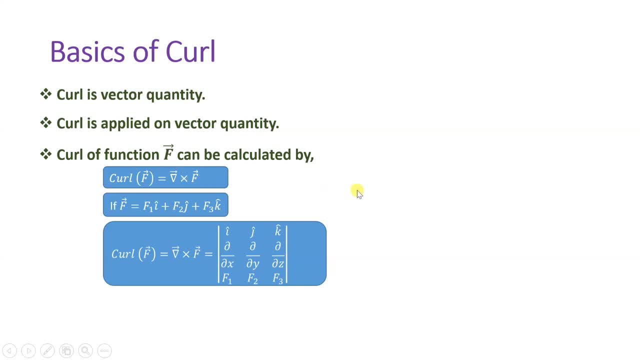 Stop Stocks theorem. now see how it explains stock theorem. so see del cross f. Curl of function f. that can be even calculated by limit Surface Del s Tends to zero Integration. Close integration: f dot dl divided by del s. 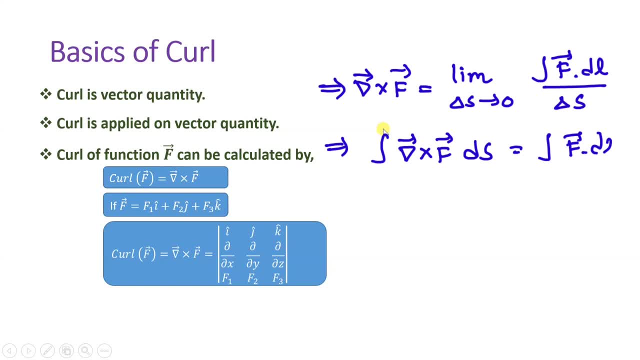 And if you do that cross multiplication again, you'll be finding Surface Integral Of curl of function f is equals to line integration of function f. So we have a relation in between surface integral and line integral by having stocks theorem. So integration del cross. 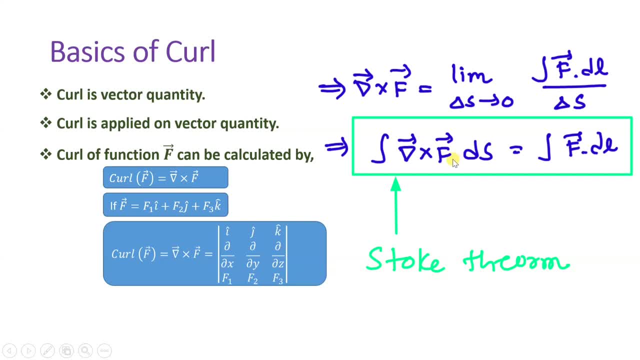 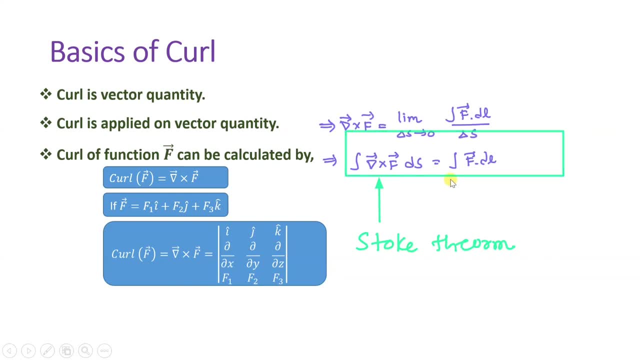 F, ds is equals to integration of f- dl. that is what Stocks theorem. Now let us have One practical example of curl So it will be more clear. See, it explains variation Of function with position and direction. So here, by using curl, we can identify variation. 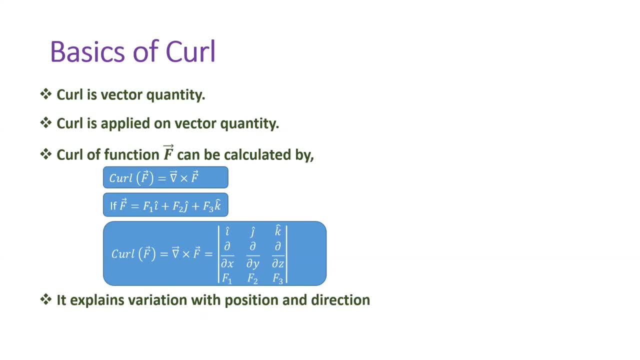 With position and direction. So let us try to understand this. See here, if we have a flow of river, you can see this is a river And flow is happening in this direction, Right. And if you place a turbine inside, So this is what. 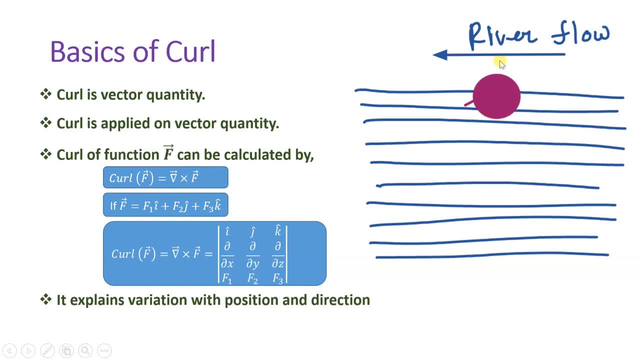 Turbine that we are placing inside. So you'll be finding When the river is flowing in this direction: upper layer, that is having higher motion, And lower layer of river, that is having lower motion. So what will happen is like when the river is flowing in this direction.